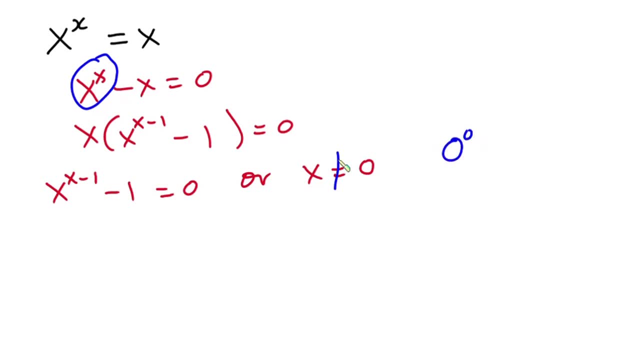 the power zero, which is indeterminate, right. So x is never equal to zero. So now let's focus on this equation. So here we have: x to the power. x minus 1 is equal to 1, and I'm going to name this equation equation star, right. So from this equation we'll be considering two cases. So we 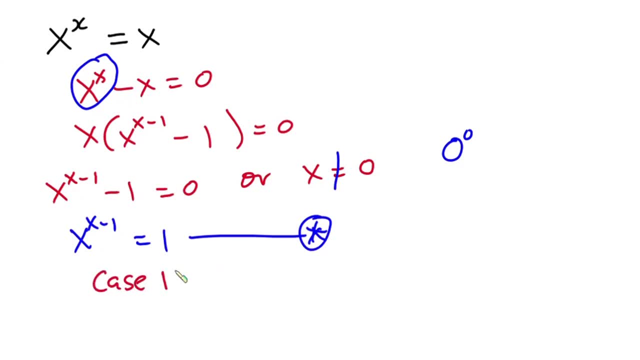 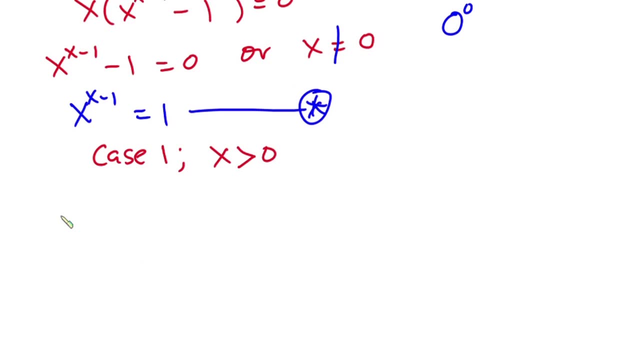 say that case one, case one, x is greater than zero. All right, so here I'm going to take natural log on both sides. So we have the natural log of x to the power. x minus 1 is equal to natural log of 1.. So from here we have x minus 1. then natural log of x is equal to natural log of 1 is zero. 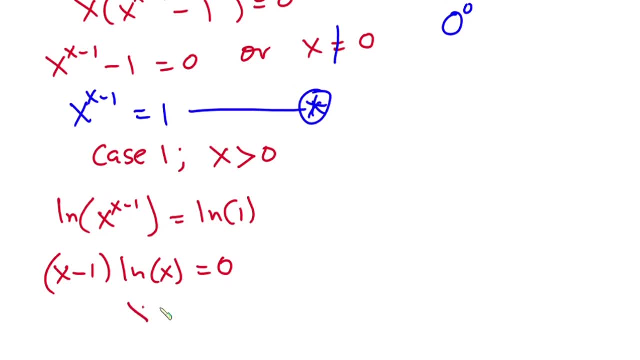 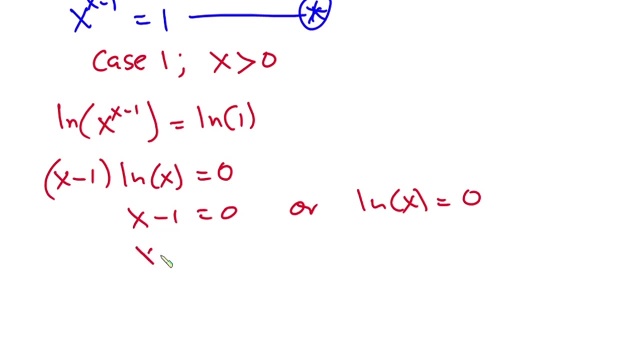 All right. so this means that it is: either x minus 1 is equal to zero or natural log of x is equal to zero. So now let's go ahead and then simplify this. So x minus 1 is equal to zero is simply x is equal to 1. or now here we have e to the power. natural log of x is equal to e to the power zero. 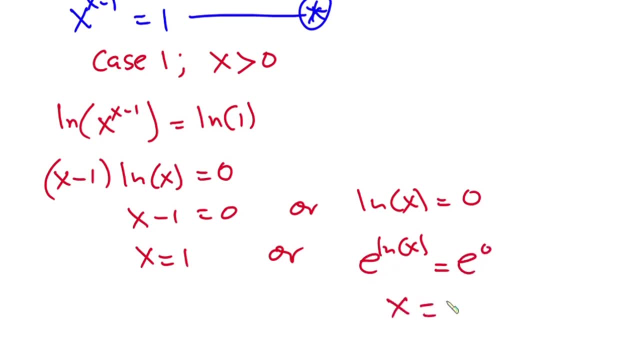 Then this is the same as x minus 1 is equal to 0. So x minus 1 is equal to 0. So x minus 1 is equal to 0.. x is equal to 1.. So either of them is equal to 1.. So let's come to the second case, which is: 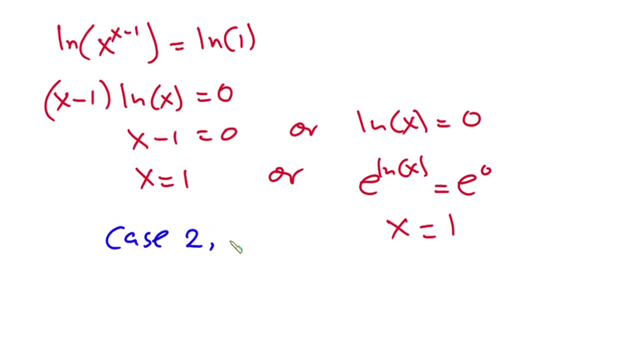 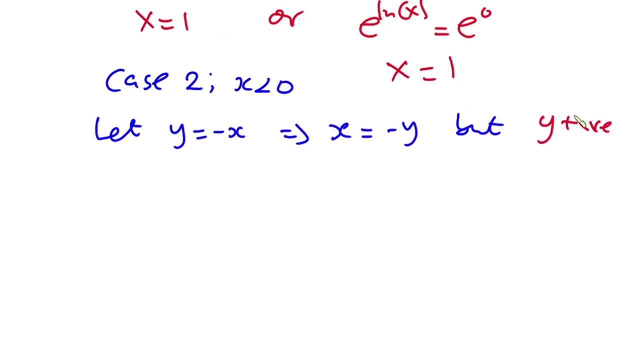 case two, where x is less than zero. All right, so from here we are going to say that let y equals negative x, and this implies that x is equal to negative y, but y is positive. So note this very well, y is positive. So putting this into the equation, which is equation star, 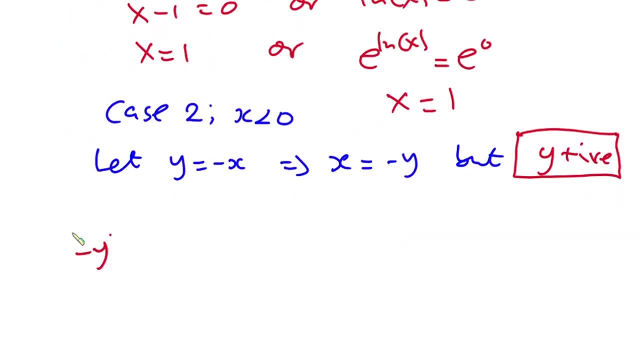 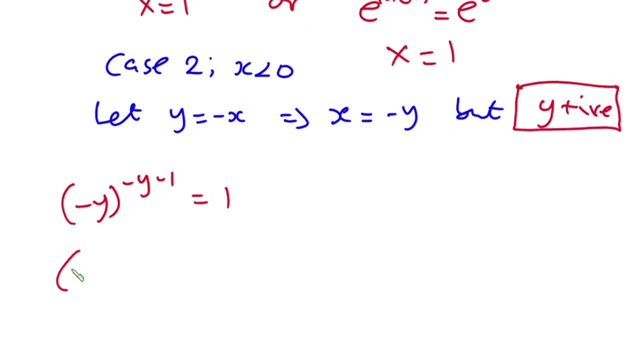 we have negative y to the power: y minus 1 is equal to 1.. Now I'm going to multiply this by negative 1 to the power minus y minus 1.. Then we have negative y to the power minus y minus 1 is equal to 1..